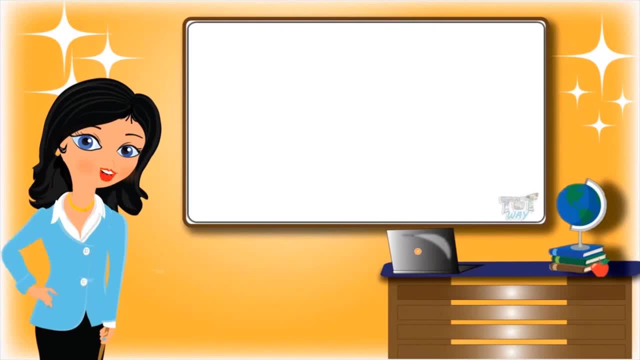 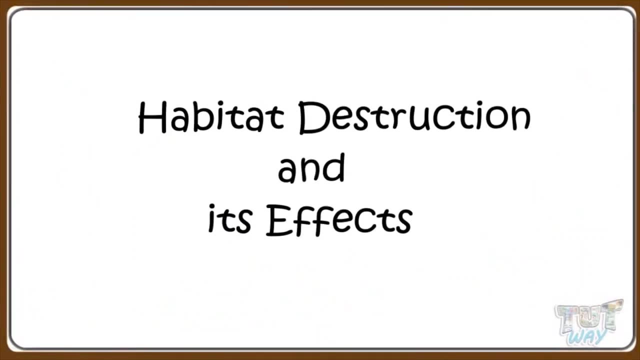 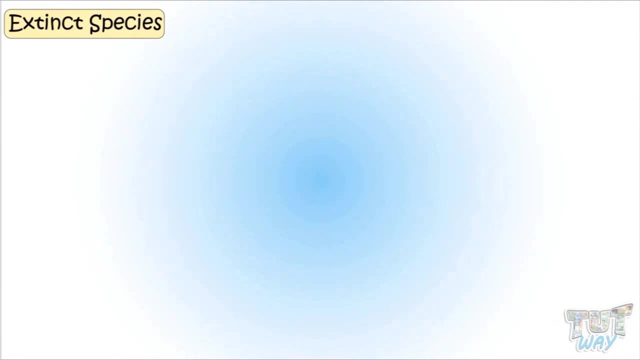 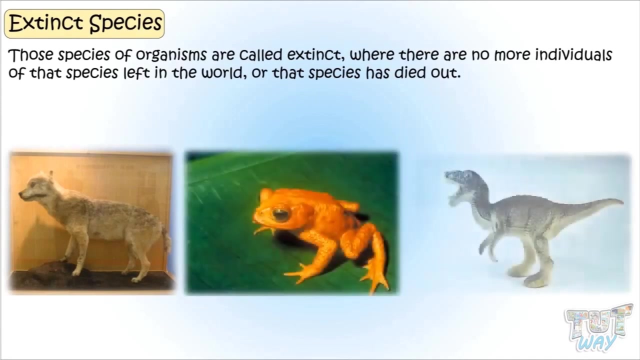 Hi kids. Today we will learn how we are interfering with the natural habitats. that is, disturbing animal life. So let's start. First of all, we will learn what are extinct species. Those species of organisms are called extinct when there are no more individuals of. 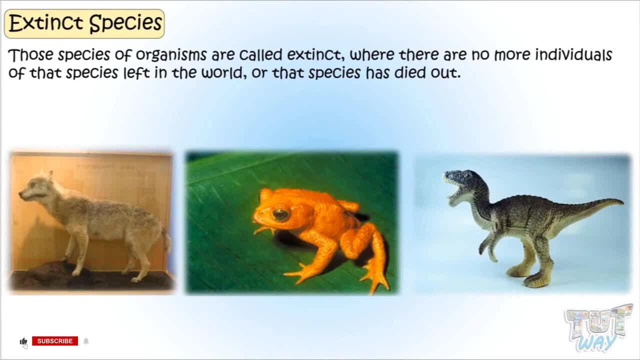 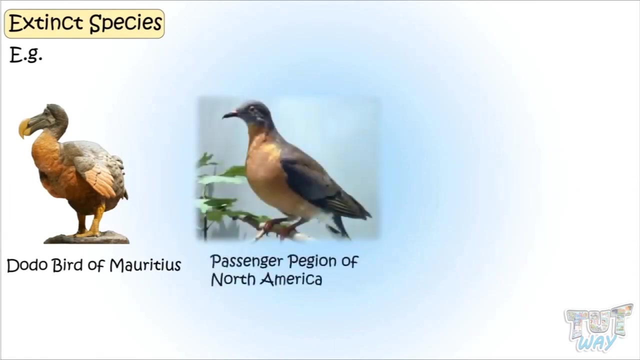 that species left in the world or that species is died out. Millions of species that ever lived on earth have gone extinct by now. That is, our earth is deprived of so many beautiful species. Now let's look at a few examples: Dodo bird of Mauritius. passenger pigeon of North America. 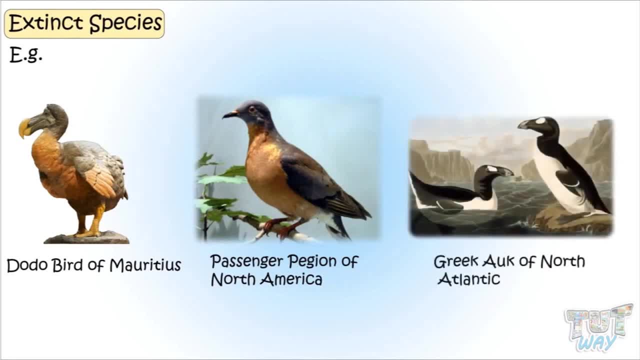 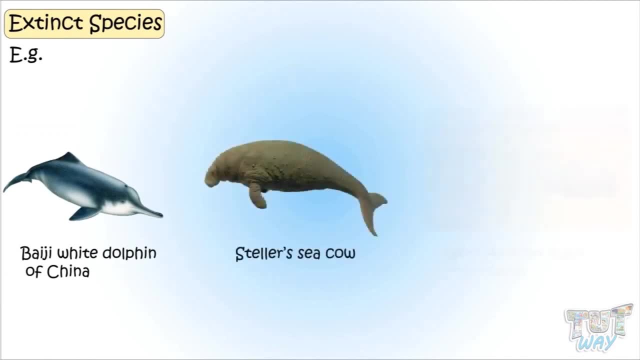 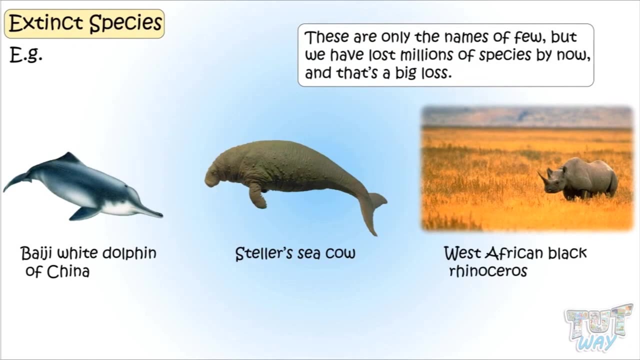 Greek auk of North Africa, Atlantic Baiji, white dolphin of China, Cellar sea cow, West African black rhinoceros- These are only to name a few, but we have lost a million of species by now and that's a big loss. 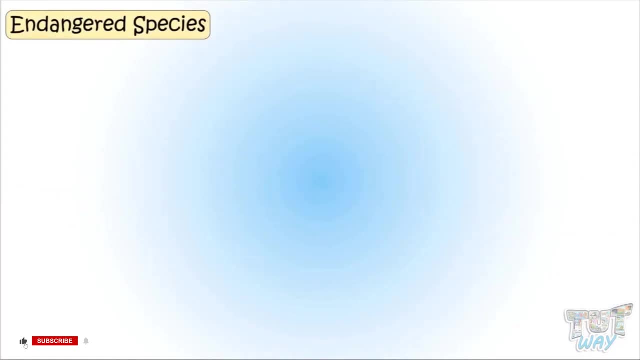 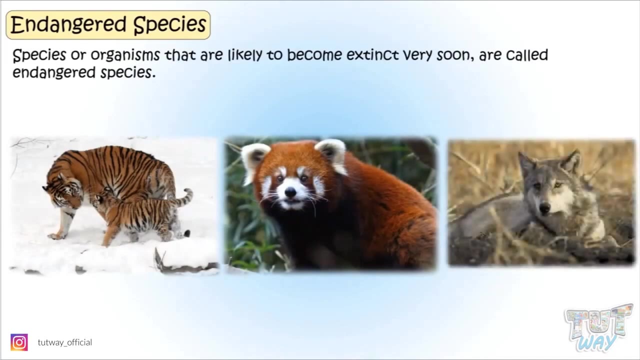 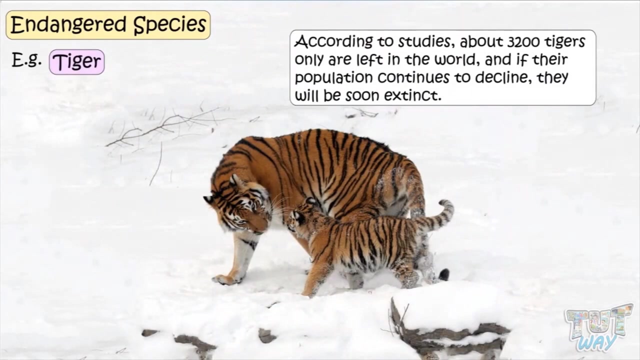 Now let's see what are endangered species. Species of organisms that are likely to become extinct very soon are called endangered species. These are the species we can save from extinction. Example: tiger: According to studies, about 3,200 tigers only are left in the world. 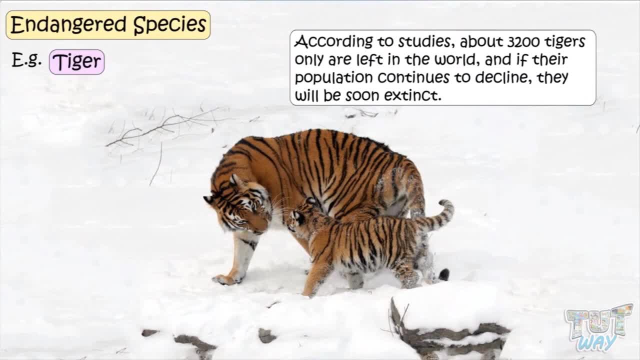 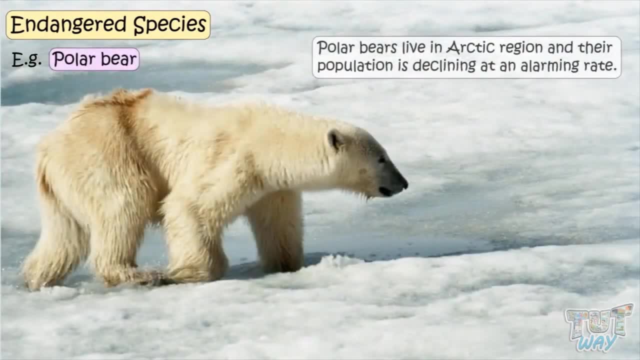 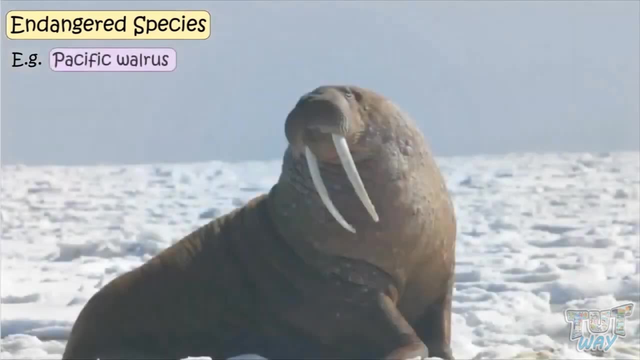 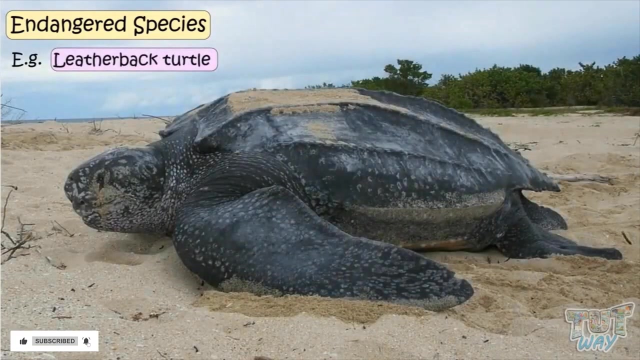 and if their population continued to decline, they will be soon extinct. Polar bears. Polar bears live in Arctic regions and their population is declining at an alarming rate. Pacific walrus, Magellanic penguin, Leatherback turtle, Bluefin tuna. 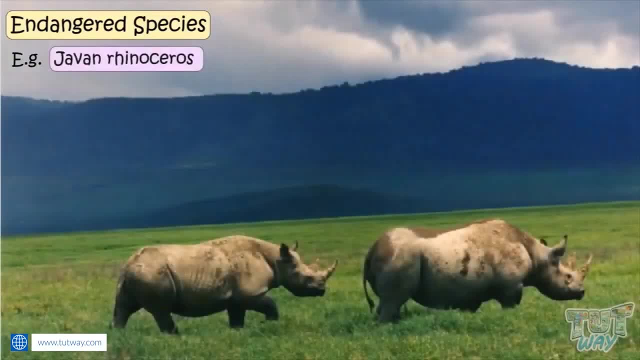 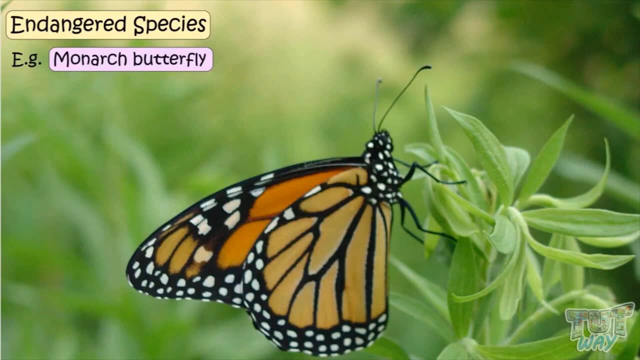 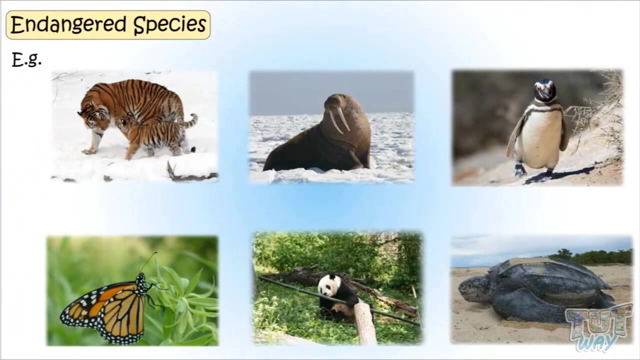 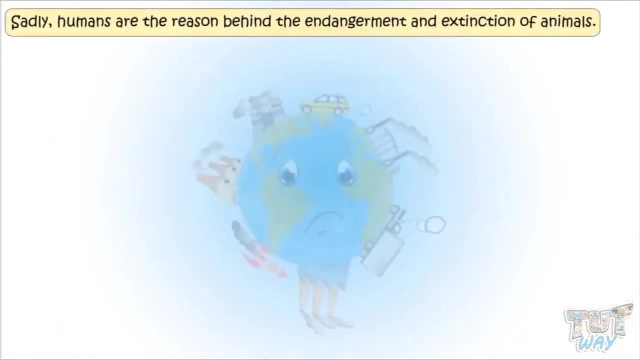 Mountain gorilla, Javin, rhinoceros, Giant panda, Monarch, butterfly and many more. These are just a few to be named. We need to save them or they will soon be extinct Kids. the most sad part is that the main reason behind endangerment and 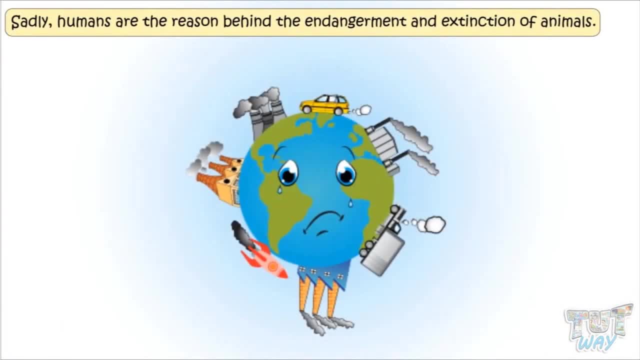 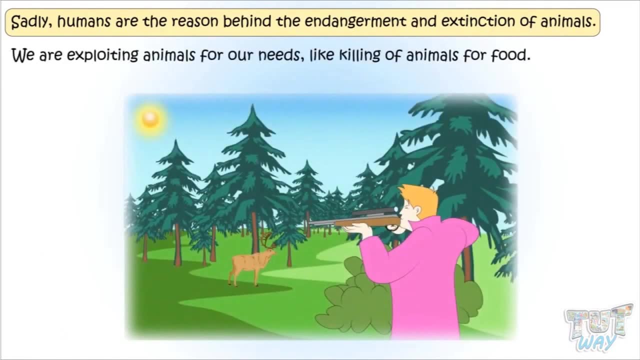 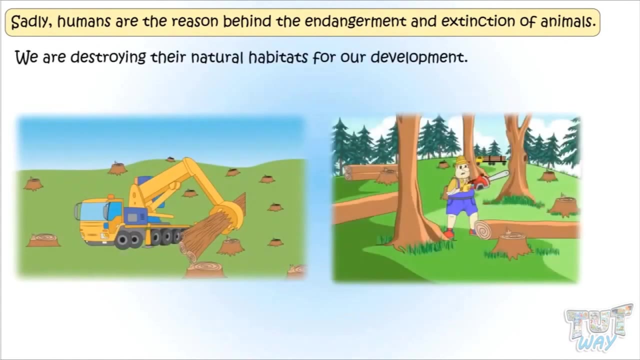 extinction of species is humans, that is, we and our development activities. We are exploiting animals for our needs, like killing animals for food, We are destroying their natural habitat for our development. clearing of forests, cutting of trees- all for wood vegetation and construction- is a great intervention in 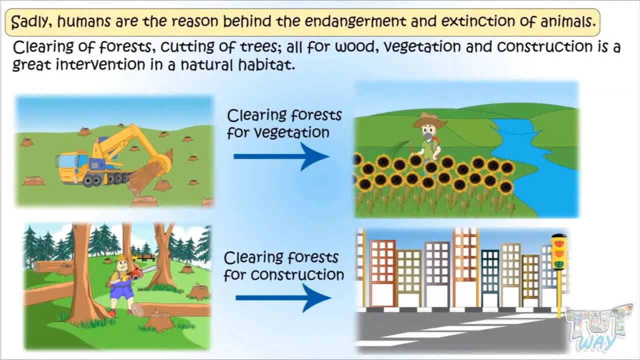 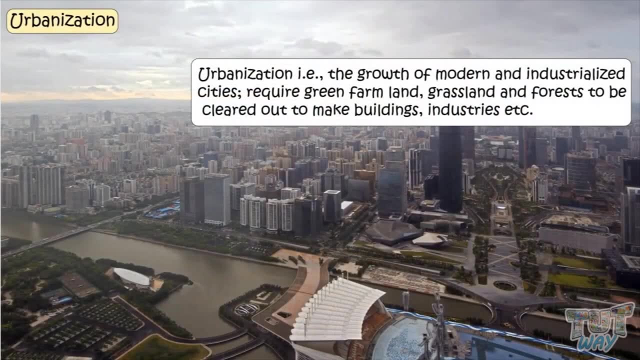 the natural habitats. It is all destroying the natural habitats of animals, because of which animals are dying out. Urbanization, that is, the growth of modern industrialized cities, all require green farmland, grasslands, forests to be cleared out to make buildings and cities, and all this eventually leads to the loss of natural habitats Ever-increasing. 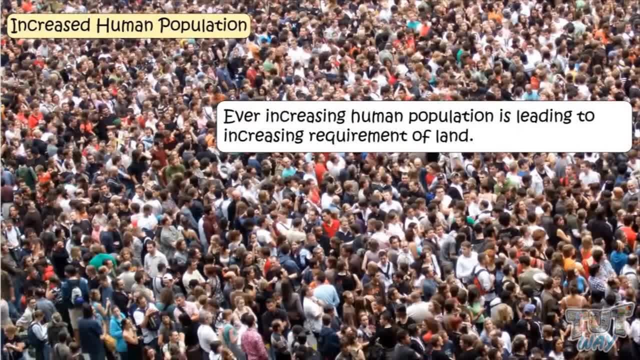 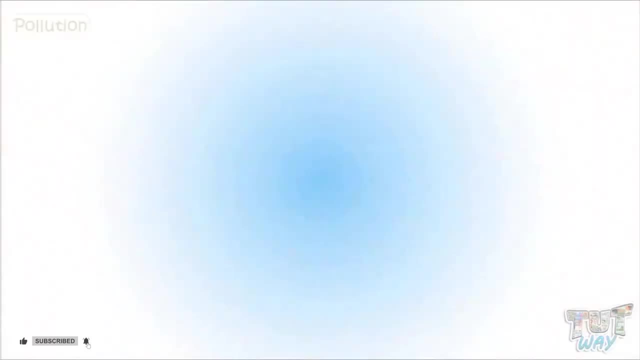 human population is leading to the increasing requirement of land, and land requirement is met by clearing out forests and grasslands, and that too leads to habitat destruction. We learnt urbanization and increasing population are leading to the loss of habitats. Another reason is pollution. Pollution is the presence of unwanted substances in our 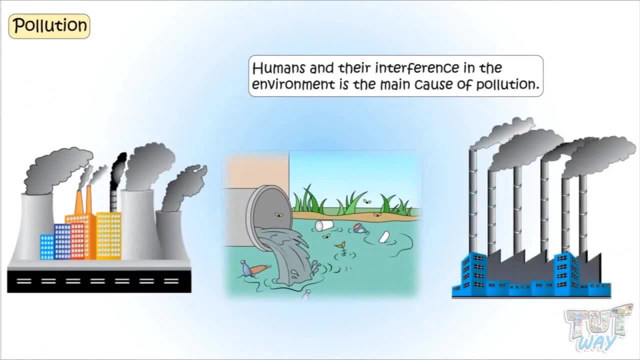 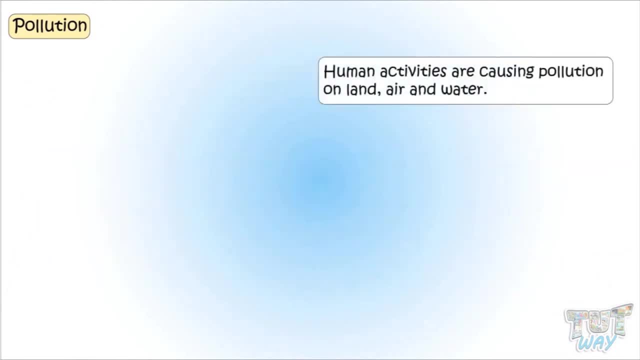 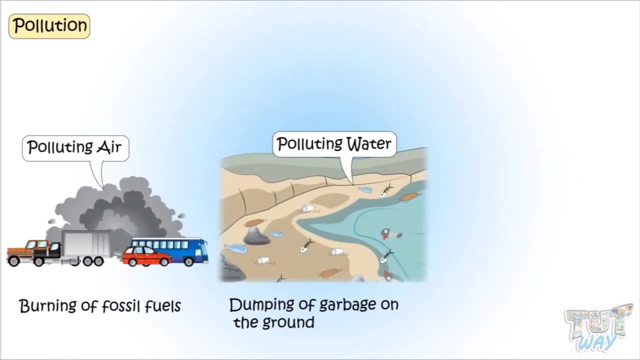 environment. human and its interference in the environment is a main cause of pollution. The Human activities are causing pollution on the land, air and water. Burning of fossil fuels, dumping of garbage on the ground, using chemicals in farming: everything is leading to the pollution of air, water and soil. 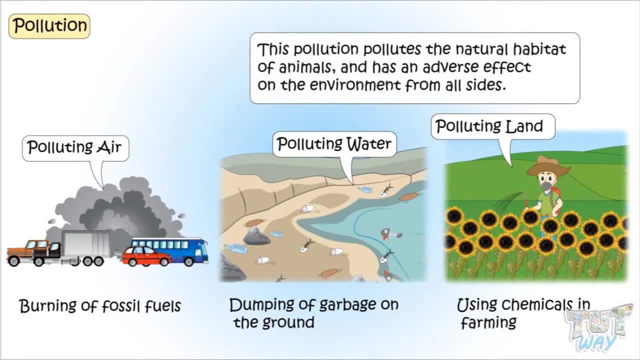 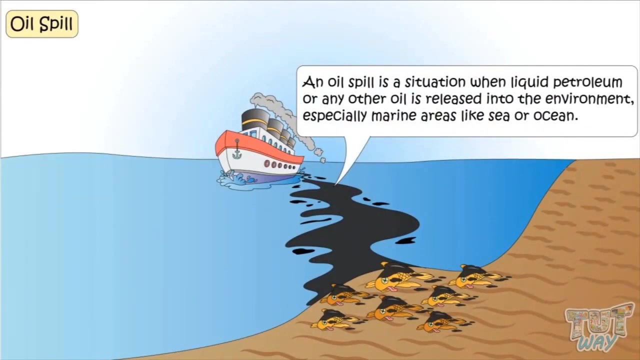 And this pollution pollutes the natural habitats of animals. Pollution has an adverse effect on our environment from all sides. All animals, birds, plants, aquatic life and humans suffer because of this pollution. The biggest example is oil spill. An oil spill is a situation when liquid petroleum or any other oil is released into the environment. 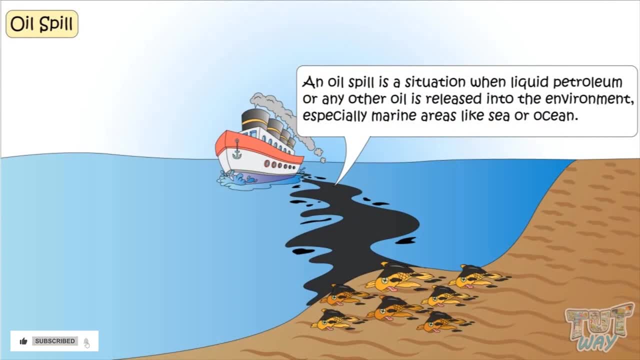 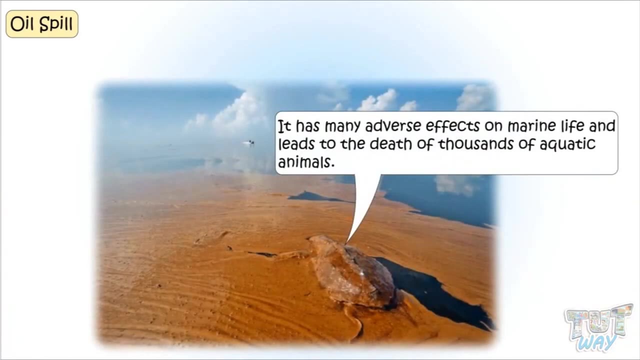 especially marine areas, that is, sea or ocean. It can be due to the leakage from some carrier ships or some accident that may have caused the pollution of the land. It has a very adverse effect on the marine life and this leads to the death of thousands of aquatic animals. 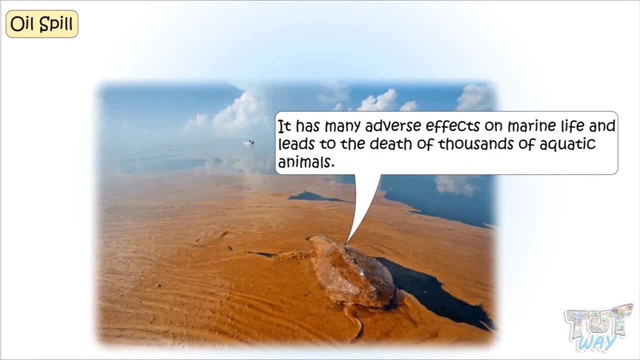 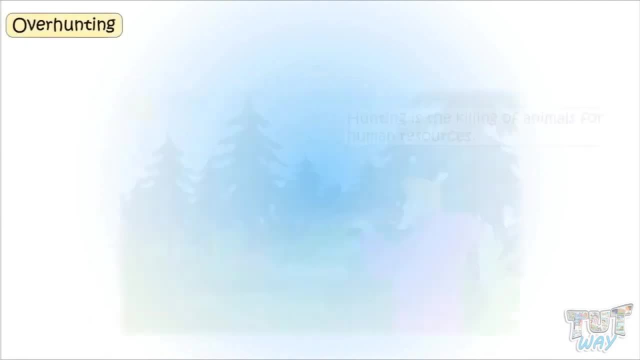 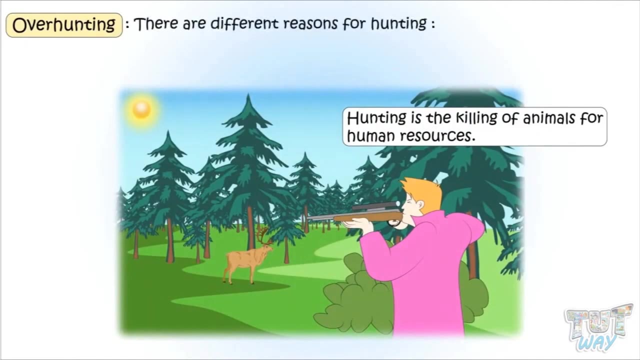 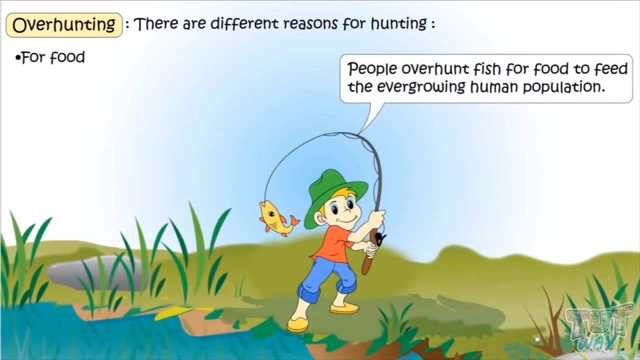 Another important reason for the endangerment and extinction of species is overhunting. Hunting is the killing of animals for human resources. There are different reasons for hunting. It can be food. like people overhunt fish for food to feed the ever-growing human population. 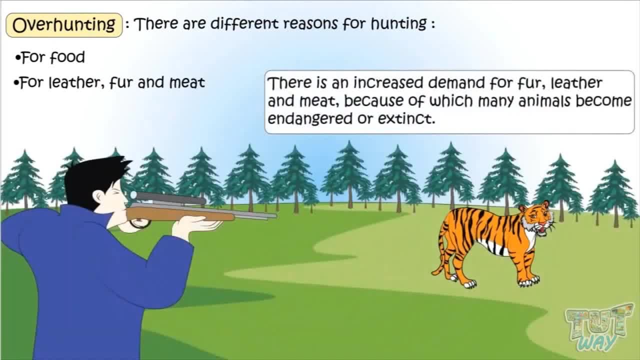 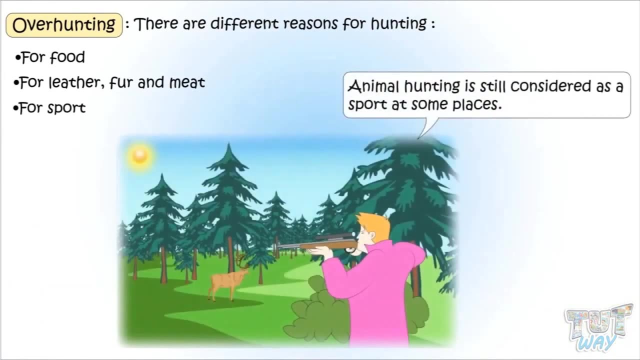 Leather or fur. There is an increased demand for fur, leather and meat, because of which many animals become endangered or extinct. even Sports- Animal hunting- is still considered as a sport in some places, Whatever the reason may be, but hunting 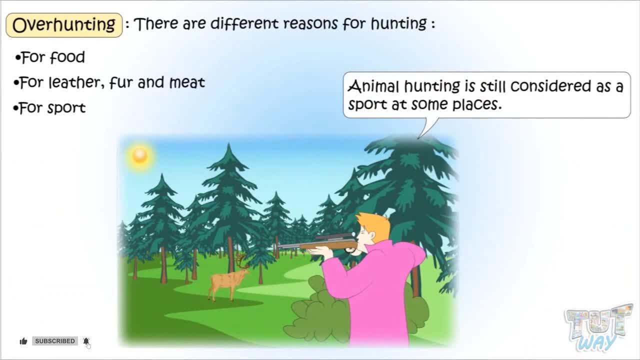 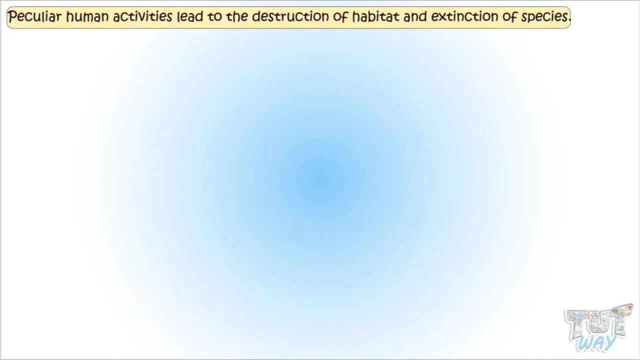 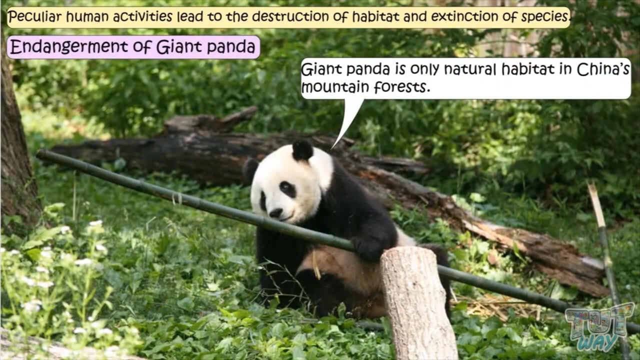 is a major and foremost threat to the declining population of many animal species. Now let's see some peculiar examples of human activities that are leading to habitat destruction and animal extinction. Giant Panda. Giant pandas' only natural habitat is China's mountain forests. Pandas prefer to live alone, that is. 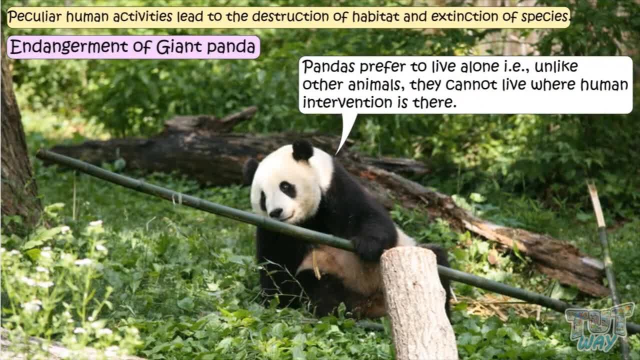 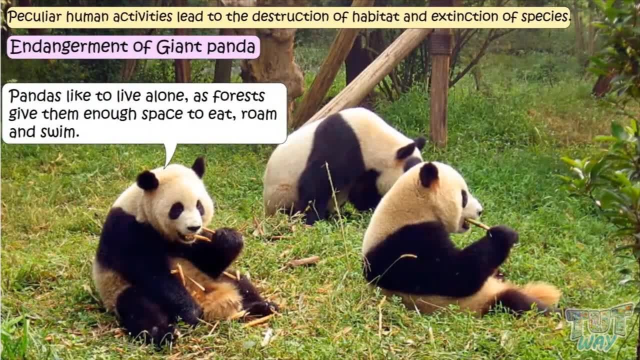 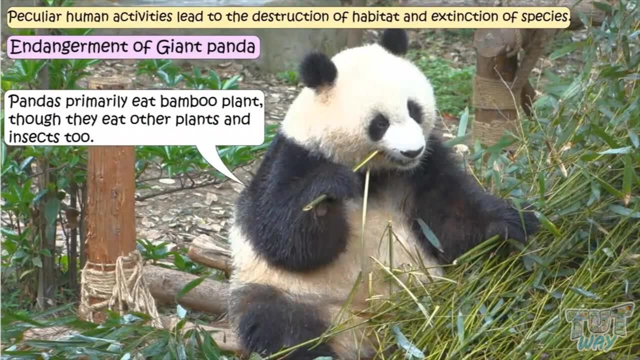 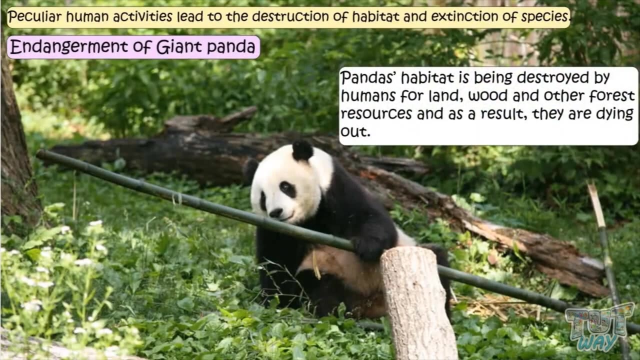 unlike other animals, they cannot live where human intervention is there. Panda like to live alone, and forest gives them enough space to eat, roam and swim, And they primarily eat bamboo plants, though they eat other plants and insects too. But pandas' habitat is being destroyed by humans for land, wood and other forest resources.